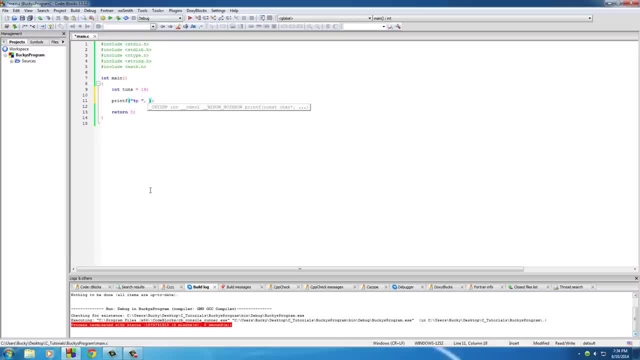 And, as you guys are going to see later on, that stands for pointer. Now, of course, if we just try to print out tuna, it's going to try to print 19, which isn't the case. We want to see where in our computer's memory this is printed out. So in order to do that, we need to use a special symbol called an ampersand. right there, You guys know what it's called. I just I don't know why I said that, But basically ampersand. and then the name of the variable says: print out the memory address. 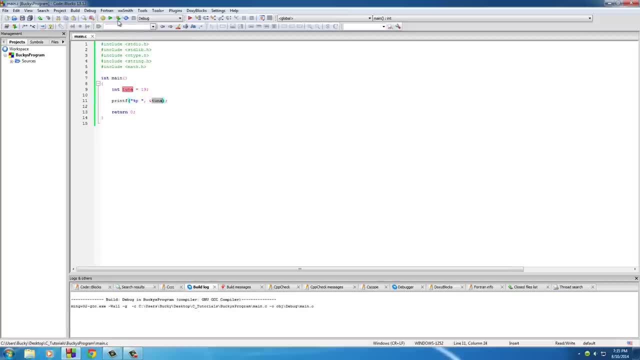 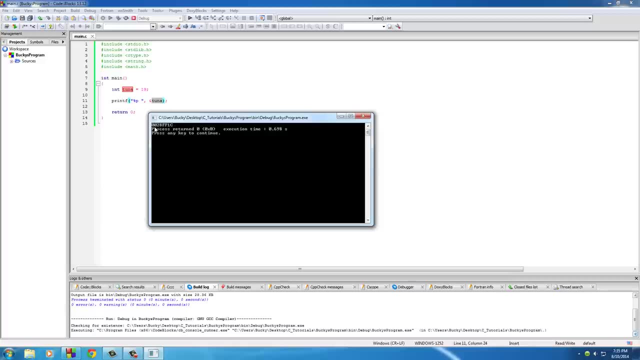 And that's where this tuna variable is on your computer. So let's do that right now. So this tuna variable is stored somewhere in our computer in memory 0028FF1C. Okay, that's a I don't know kind of interesting Bucky. I mean, computers obviously store variables a little bit different than we think they do, And the reason for this is because if we just try to use that memory address in our computer, 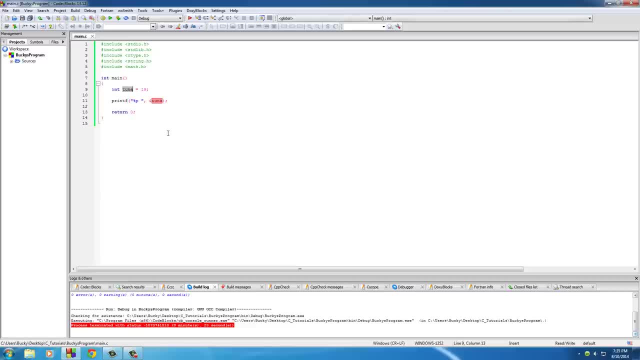 Instead of this variable name. I mean, it's kind of hard to work with, It's kind of hard to remember and understand. So what C allows us to do is use this name instead. Okay, cool, But who cares? You know who cares what happens behind the scenes in our memory? Not important, Kind of interesting, But who cares? Let's skip pointers for now. Well, just a second. There are some instances where you need to actually work with the memory address of your computer, And in about three tutorials, 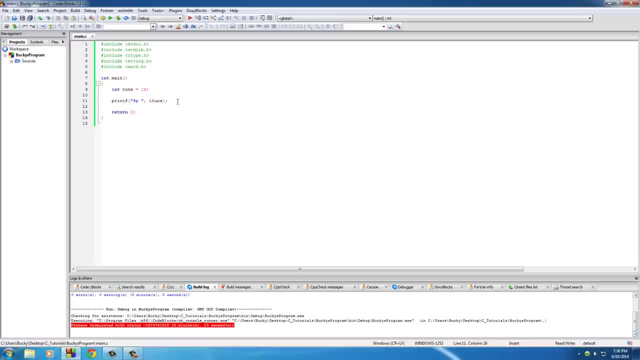 To see exactly why. But for now, Let me display a couple things to you. So what we can do Is I'm going to be building a little program in this tutorial That basically shows you guys the address, the name and the value of a few variables, including pointers. So the first thing Is we're going to be printing out the memory address, just like we saw, And then the name of the variable, which in this case would be tuna, And then the value of it, which would be: 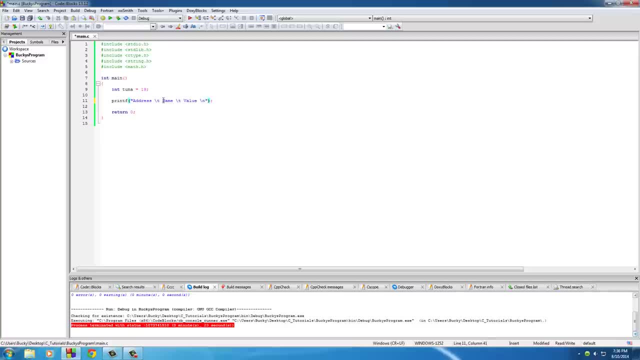 19.. But it's going to be a little cooler than that. So of course, Well, I guess we can. Let's just keep that line simple. We'll keep this program really easy to understand. So in this print statement down here We'll do it first for this tuna variable. So of course the first thing we want to print out is percent P And then tab that, And then the name, of course, is just going to be a string. This is just going to say tuna. So 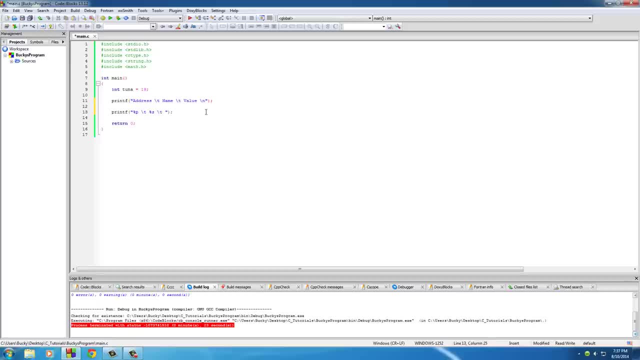 Percent s tab, And lastly the value, which is percent D, To kick it to a new line. So we'll print out tuna, The address of tuna, which is going to be zero, zero, whatever tomato, tomato. Then the name, Which is tuna, And then the value And, of course, just like before, whenever we want to print out the value of a variable, Just use this name on percent D, Run it and check it out. So now we can visualize this a little bit better. 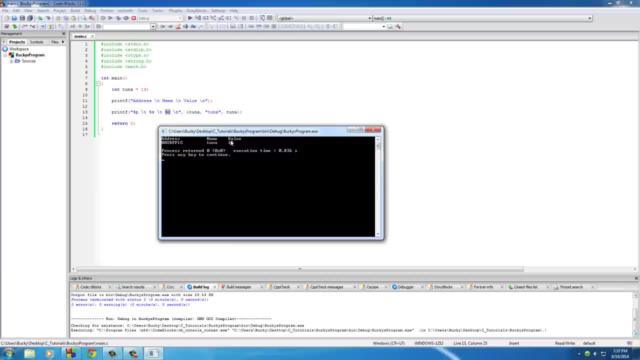 So this tuna variable Has a value of 19.. And to us we can just use the word tuna, Because C is pretty cool And it allows us programmers of stupid human beings to use simple names for stuff. But of course there's not just a random spot in your computer's memory named tuna Waiting to be filled with some number. So we made this. But what your computer actually sees Is this space right here. That's a space that was waiting, And whenever it actually uses 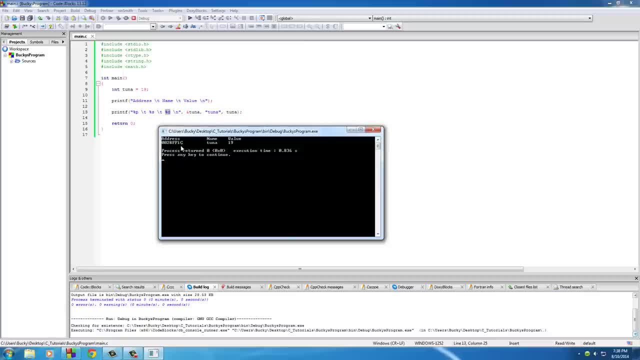 This variable. That is the address that it has to go to. Alright, So that was pretty interesting. So what the heck's a pointer? Well, we know that this right here is a memory address, And what a pointer is Is a special type of variable That can hold this address. Because, look at it, Zero, zero, two, eight F, F, one C. Well, we can't just store it in like an int Because it has characters in it. We don't really want to store it in a string Because it's kind of 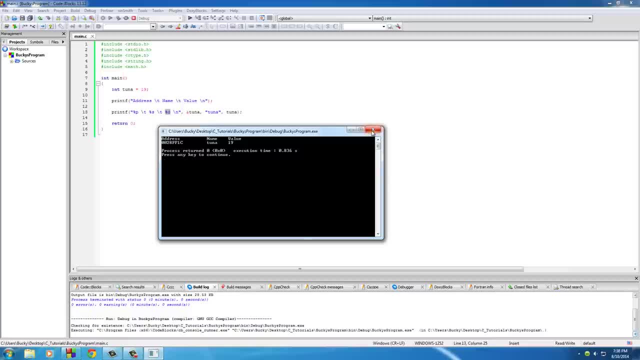 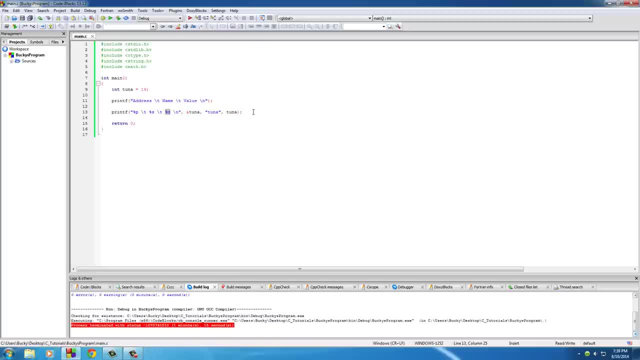 Like a mixed up, Has numbers. So we need to make a special type of variable Whenever we want to store these addresses, And those variables are called pointers. I'll show you guys how to do that right now. So in order to make a pointer variable, You type what data you're going to be storing, Or we'll store a pointer to this one Which was an int. So put int And if we just type the name after it, It's going to be a regular integer variable, But we say we want to store the memory address. 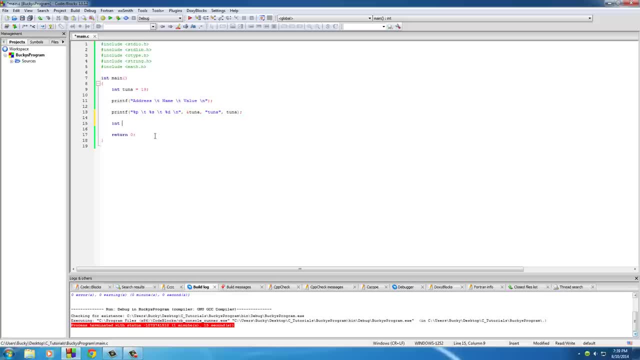 Of an integer variable. So if you type the asterisk, It's above the A on your keyboard. What this is basically telling C Is we're going to be making a special type of variable To hold a memory address Called a pointer. Now the truth is, you can name your pointers Anything you want. You can even name it two and a two, But it's common practice Among programmers To begin all pointer names With a lower case P And then type the variable name That it's pointing to, And that's just So. later on, 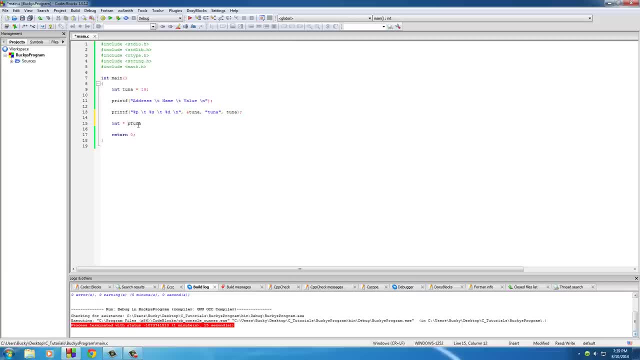 You can see, Okay, this P tuna Is a pointer to tuna. You know, just common sense stuff. So of course, This isn't going to be holding the actual integer, It's going to be holding the memory address. Now we already know How to access the memory address With an ampersand And then the name of the variable. So now what we can do Is we can use this P tuna Interchangeably whenever we would have used this, And I'll show you guys that right now. 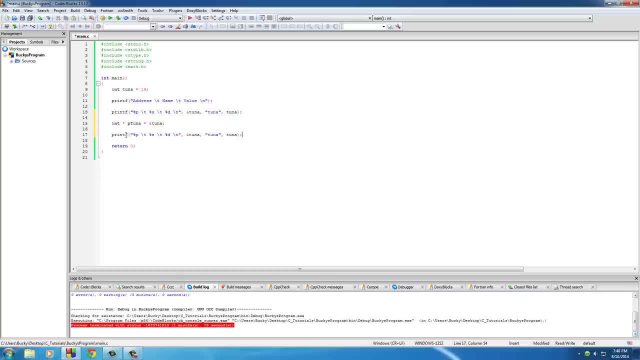 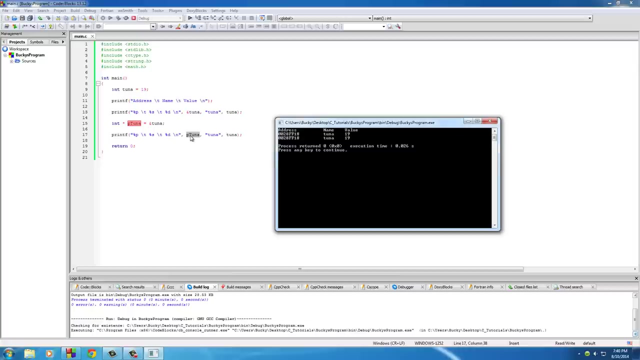 So let's print something else Out right now And we'll just change this one Right here. I guess I'll type it out: P tuna. So what this line Prints out And what this line Prints out Is essentially the same exact thing, So we can now use this variable P tuna, Instead of accessing The memory of this Directly. 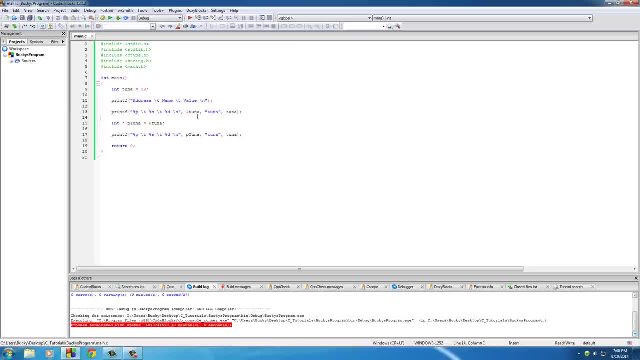 And I know you guys are saying, Okay, That still doesn't explain Why I would ever need a pointer. And for right now, We kind of just need to understand the basics Before we learn about things like How arrays are kind of pointers And the heap And all that crap And how to make cool Expandable Applications. But for right now, As long as you understand this, You'll be good to go. So the one other thing that I want to do, Just so this sticks in your brain, Is this: